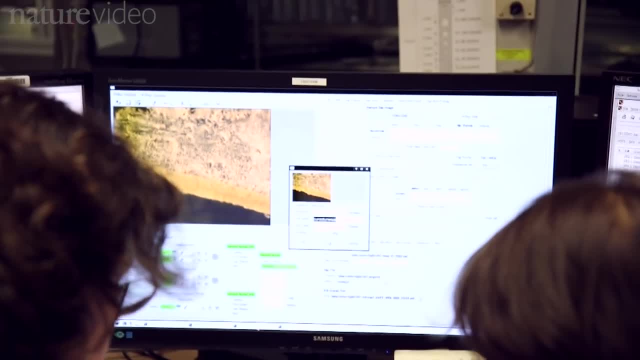 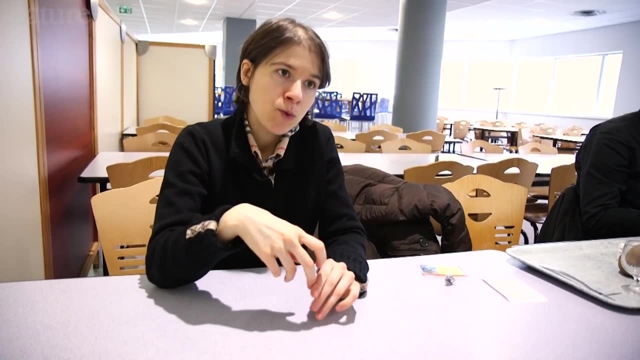 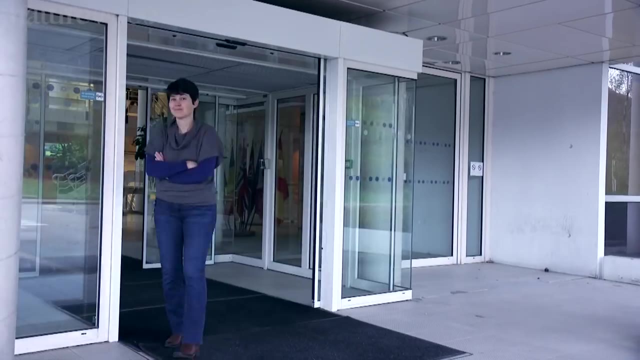 color is changing when paint is. What are the chemical reactions? So this afternoon we are going to study a series of fragments taken by the painting screen By medical threatens. We have about 8,000 scientists coming every year to the ESRF from all sorts of fields. 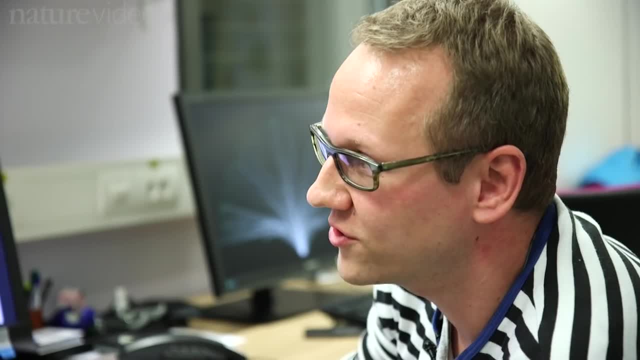 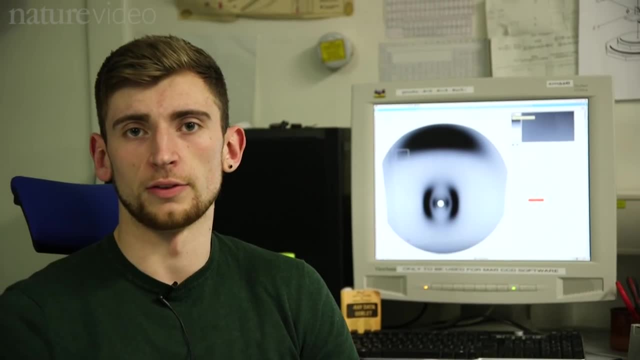 physics, chemistry, biology, Basically the structure of this electrode. here Some gas absorption on metal, organic framework, Material science, nanoscience, Liquid crystal phases, Metalloproteins by X-ray absorption and emission, spectroscopy. Museums bringing precious artifacts. 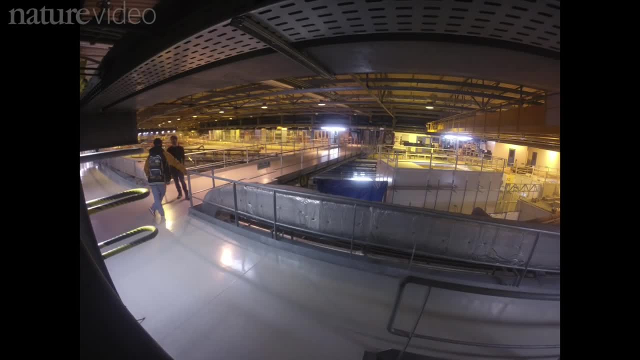 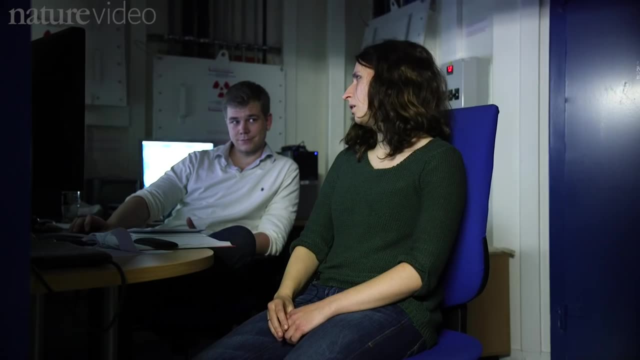 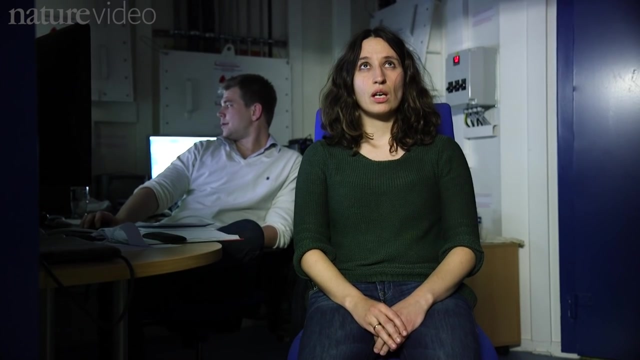 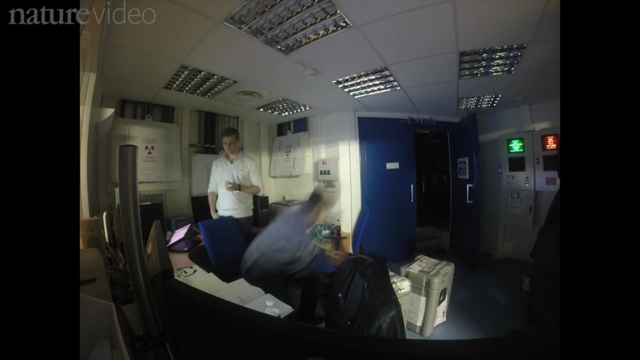 We have paleontologists, So it can be a lot of people here. So now it's half past seven. When did we start with this project? After lunch, After lunch, So I think it took us now five hours to measure one data set. We have 90. 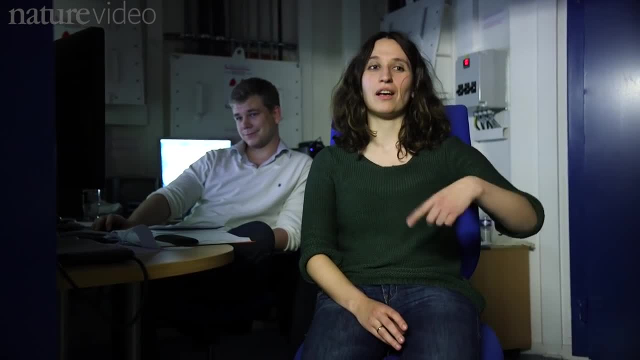 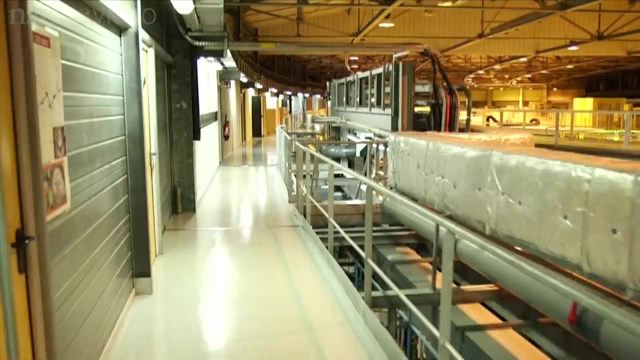 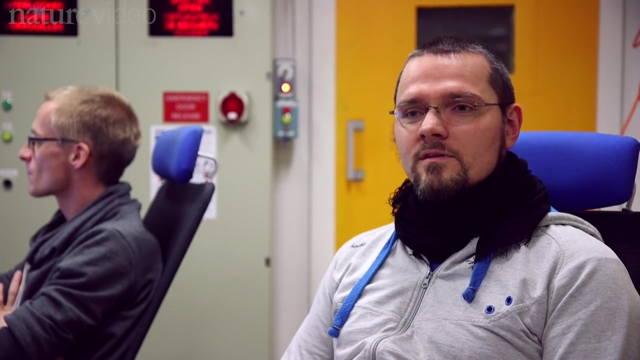 crystals left and we will check them, Crystal after crystal. How long will that take? Till tomorrow morning Nine AM Here and I? we are the night shift. We are working here from seven o'clock in the evening to eight o'clock in the morning. Beam time is expensive and rare, So we use every minute. 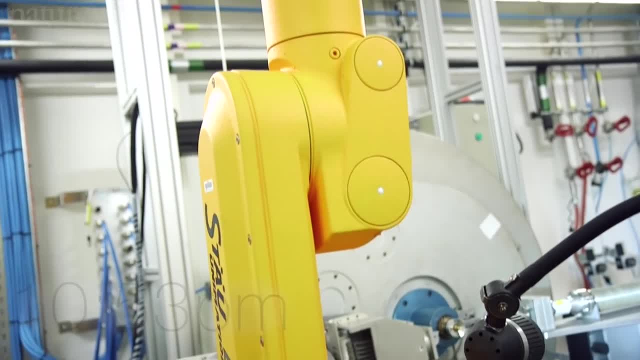 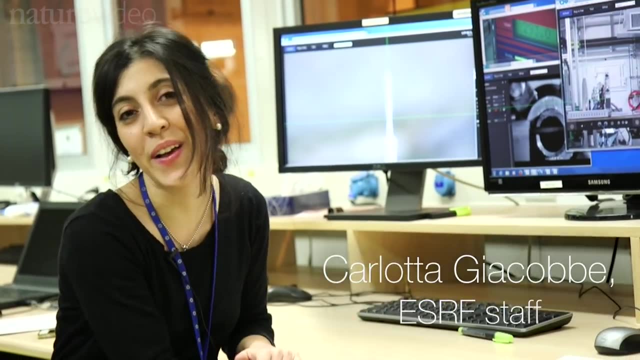 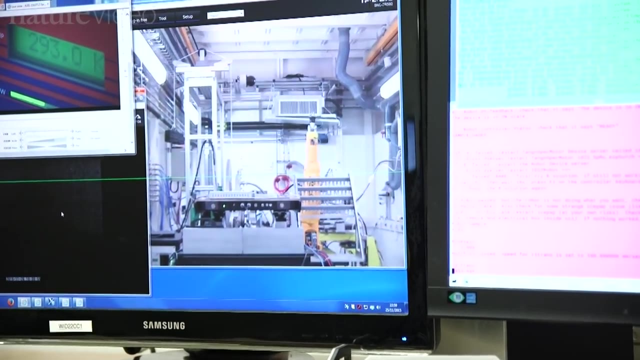 we can and we watch every step the machine does. So we are here just to check that the robot is working and is moving. Then we can go on. So here we can. we'll see if the robot is changing. sample See. So what are you looking for? 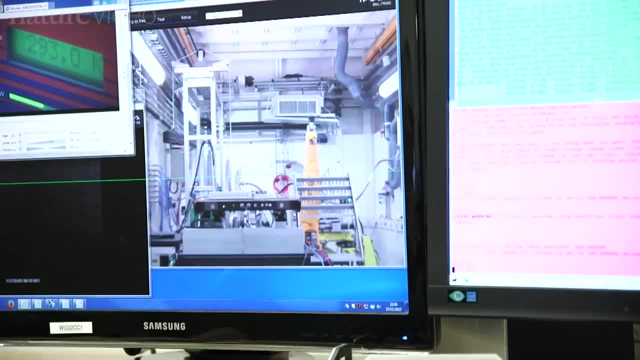 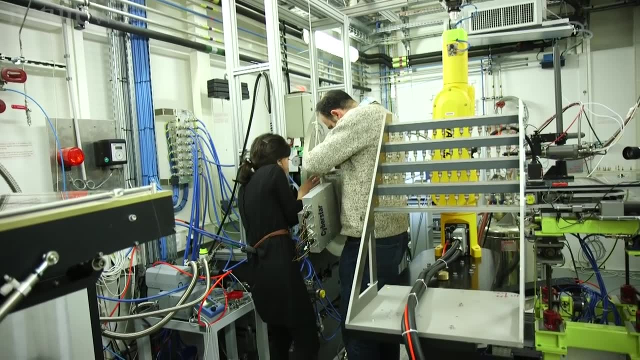 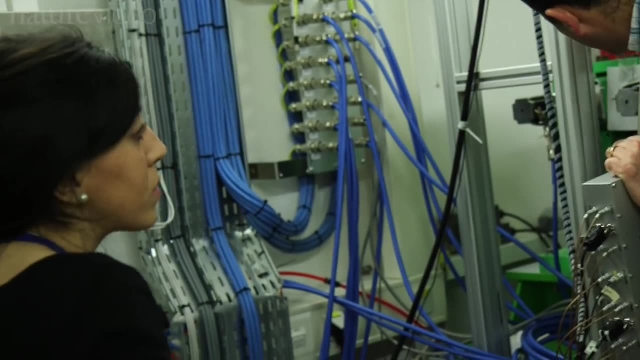 No, Wait, it didn't work. I think I have to go inside and check. See this cable. I don't know What time is it. It's too late to call him. It's four past eleven. We will lose the night. 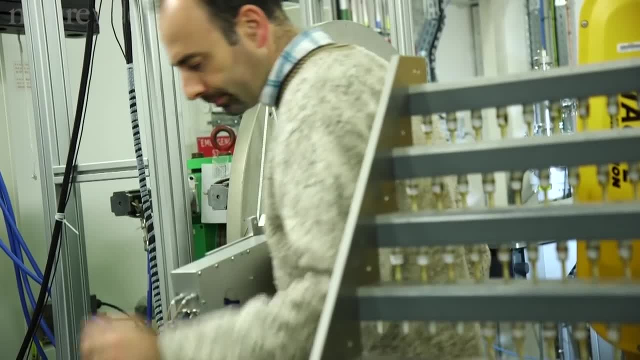 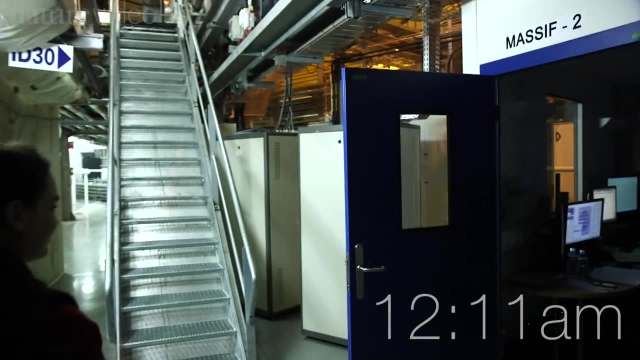 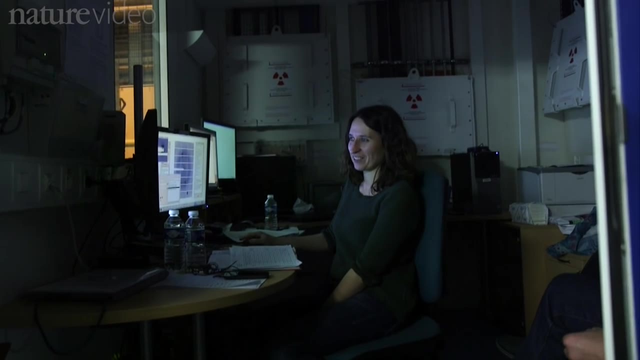 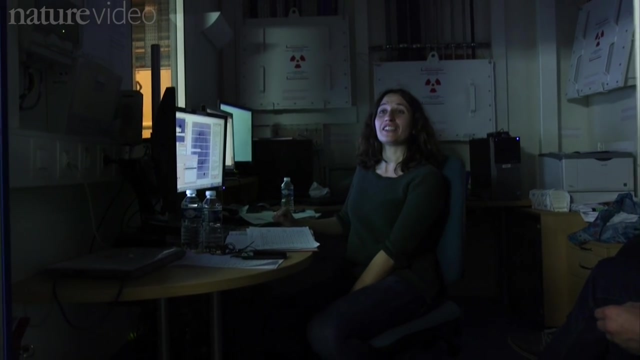 Okay, Okay, What to do Tomorrow morning? You guys are still here, You too. What's been happening, What happened? So we are very happy We could measure another data set for a mutant where we had no data set before. 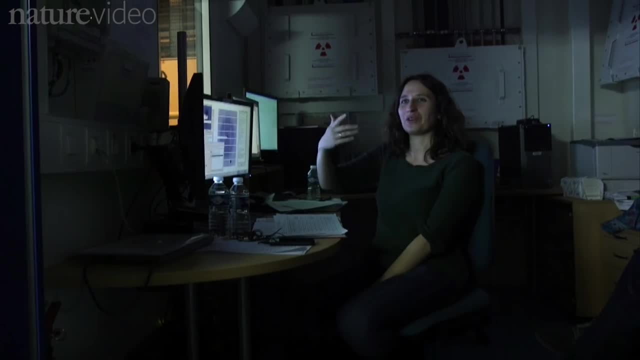 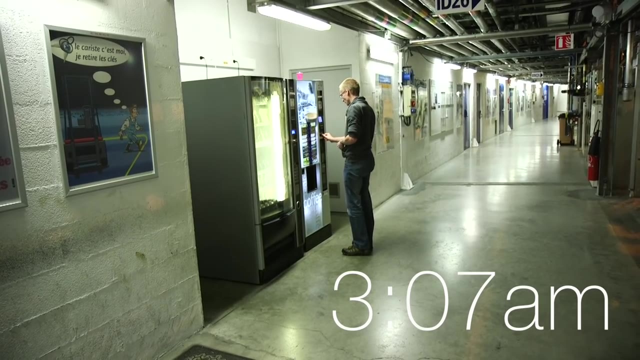 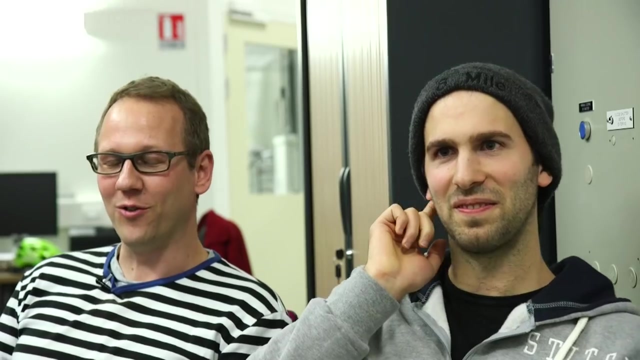 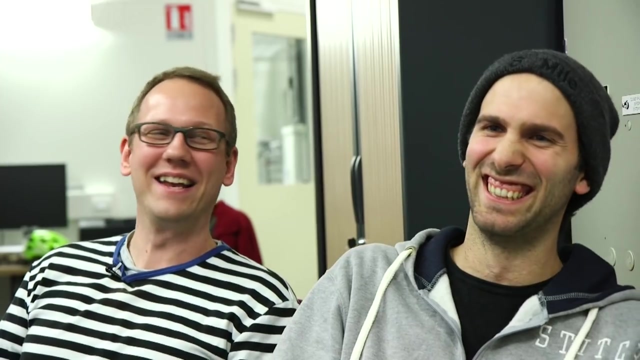 Yeah, Yeah, Yeah. So we are going on checking the next person. I am Peter Stain Janssen. I'm from the Technical University of Denmark, From the it's called. sorry, I forgot our name. I'm too tired. 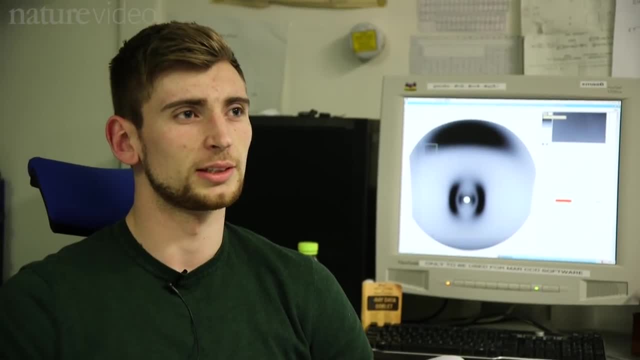 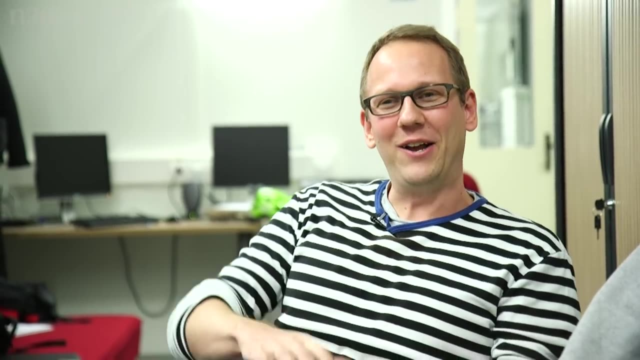 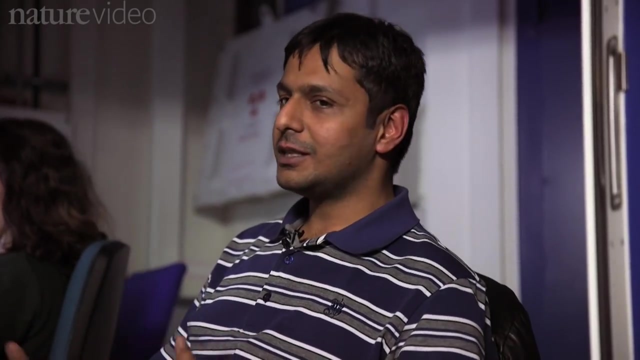 I got up at 6.30 yesterday. technically, Yeah, We are quite tired, but also we are kind of riding on a high of success, Because I'm tired but the data are interesting. so If every now and then there is something which is exciting, you know you're again on. 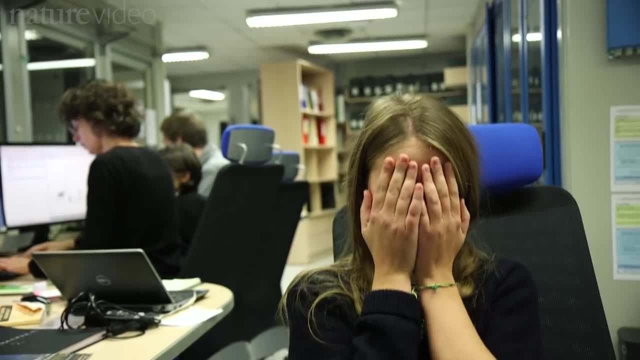 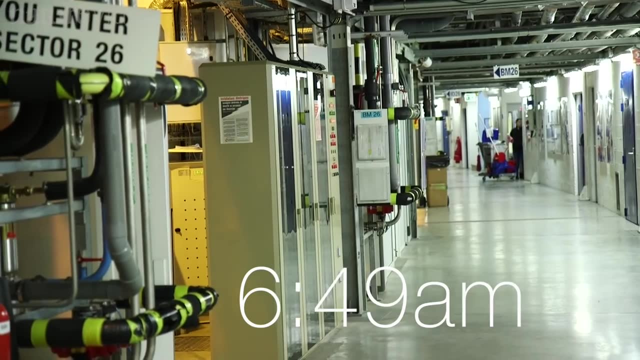 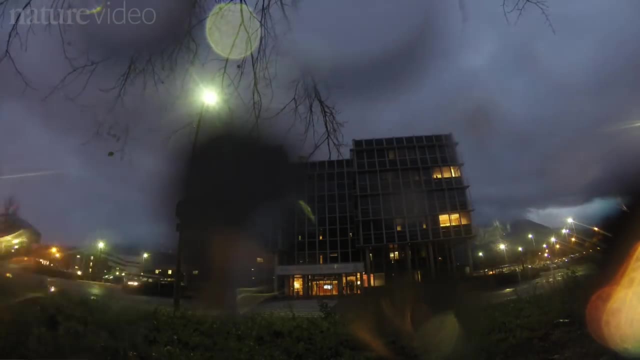 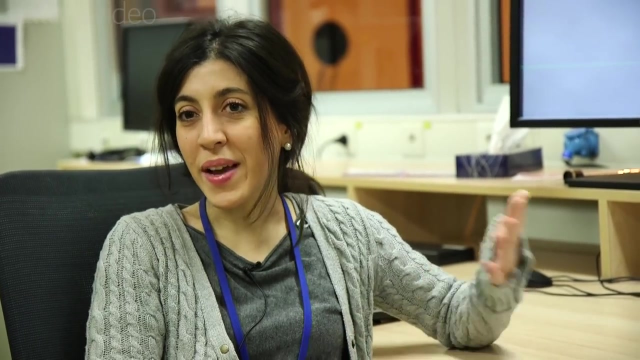 Now I cut this one. It was horrible. This is the worst timing to speak now because I'm tired. So yesterday night we had a problem, So this morning I called the engineer. We fixed this problem. So now we are just here waiting for seeing if it's working. 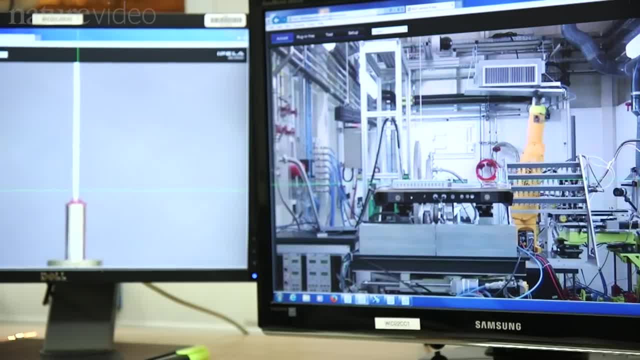 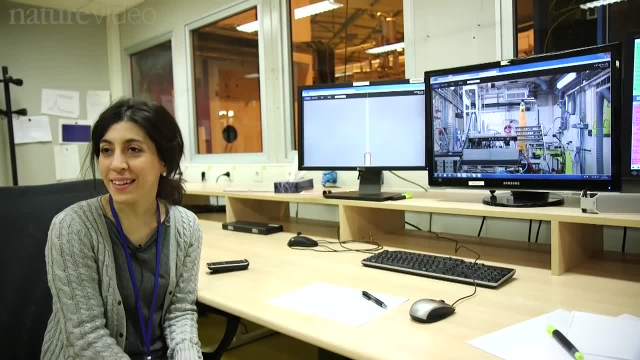 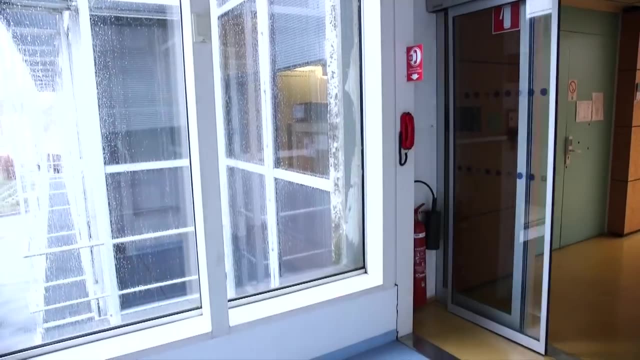 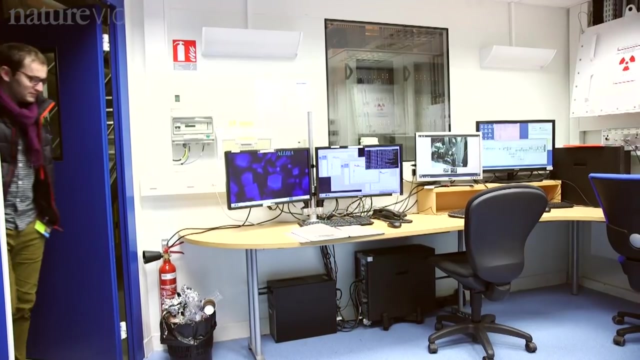 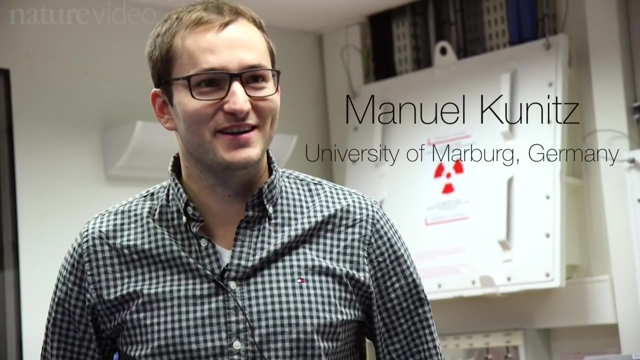 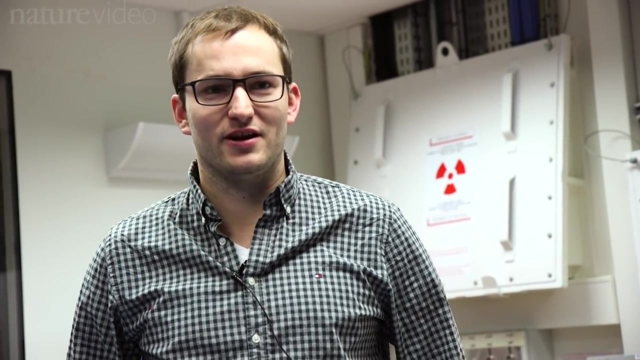 Okay, you see the arm moving. Okay, so it's working. I'm quite relieved now, So experiment can start again. Yay, Well, the crew that worked here before us, the team they just left a couple of hours ago. Now we are here and working on probably completely different projects, And now we 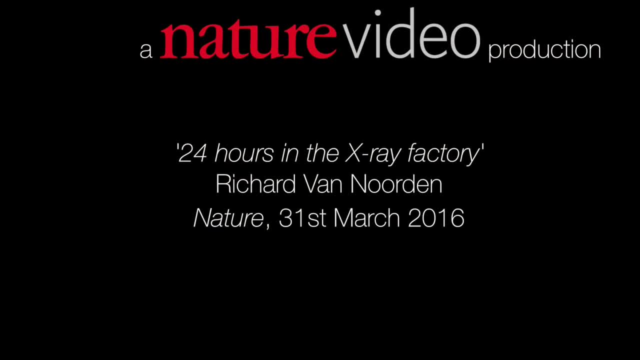 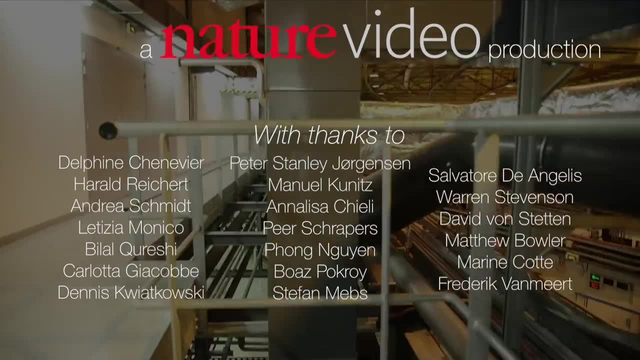 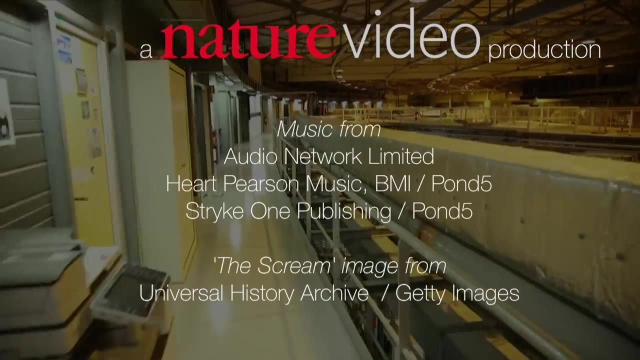 have 24 hours of beam time. Wow, we are so tired. Thanks for stopping by, Thank you. Thank you, Josh. Thank you very much, Kelly. Thank you, Thanks, guys, That was great, Thank you. Thanks for having me.